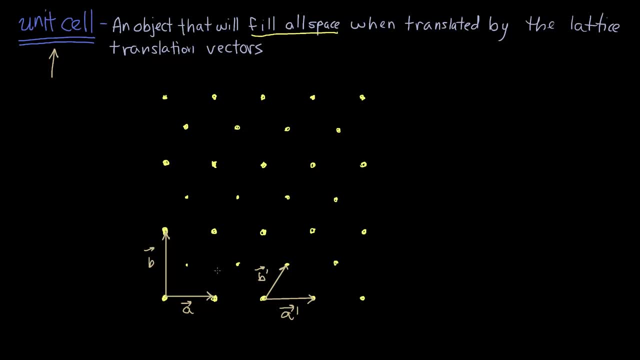 We'll construct a unit cell around these points. It's possible to have multiple unit cells for the same points. the same way we can attribute multiple lattice types to these points. So the first unit cell we could see here might be this one. I'll highlight it in what may be blue. 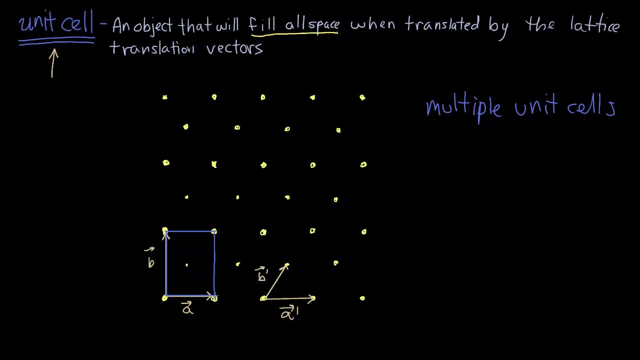 So this cell we would call a centered rectangular cell And if we use the lattice translation vectors B and A, And if we use the lattice translation vectors B and A, And if we use the lattice translation vectors B and A, We can move this cell around to fill the entire lattice infinitely. 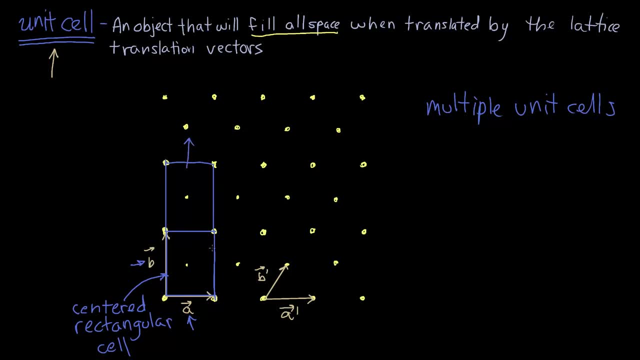 And you can see how this can keep continuing. if we move it to the right And above, we can start to fill space And you can see there would be no gaps. That's very nice. That's very crucial. We're going to fill all space with no gaps. 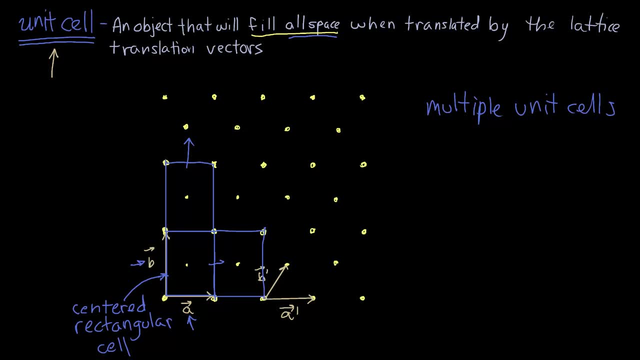 We can also draw a unit cell down here. We can also draw a unit cell down here. I'll draw it right here. I'll use a different color. I'll draw it right here. I'll use a different color. I'll use a different color. 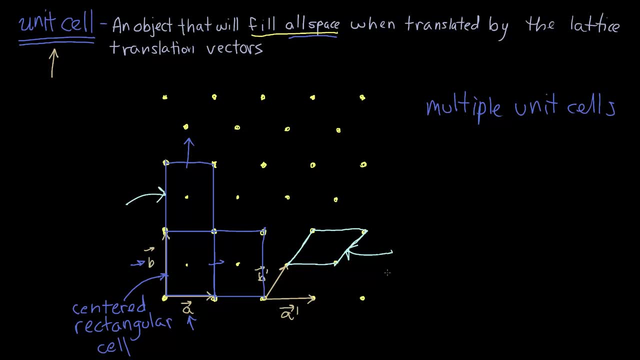 And the crucial point to note here is that we have two unit cells, but they are not preferred over one another. but they are not preferred over one another. The choice of a unit cell is arbitrary. It's up to the convenience of it. 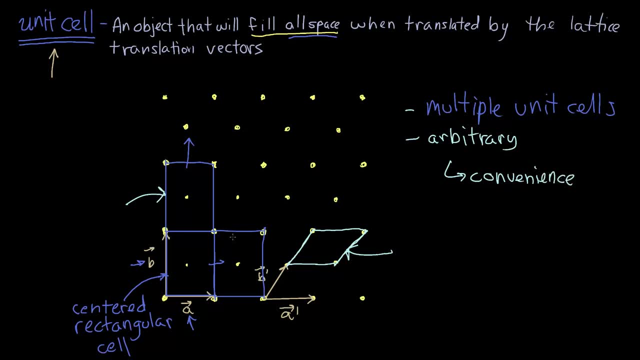 It's up to the convenience of it. So a particular problem may be. So a particular problem may be better worked out by using the centered rectangular cell than this parallelogram cell, than this parallelogram cell. This cell in particular also has a name. 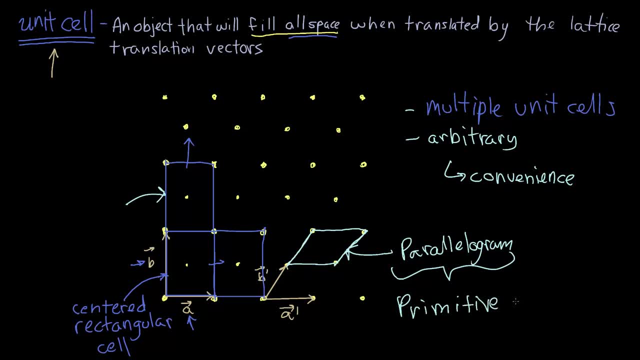 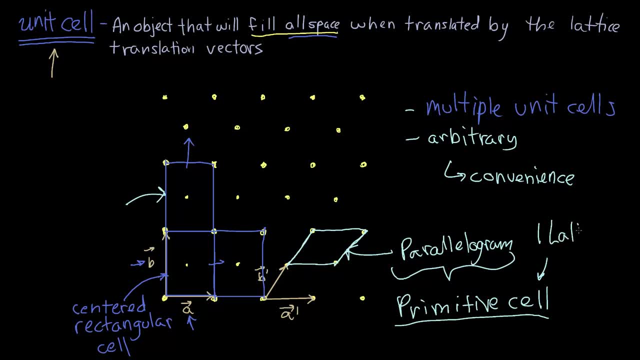 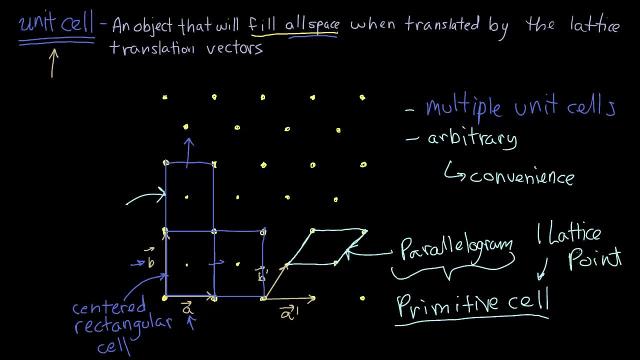 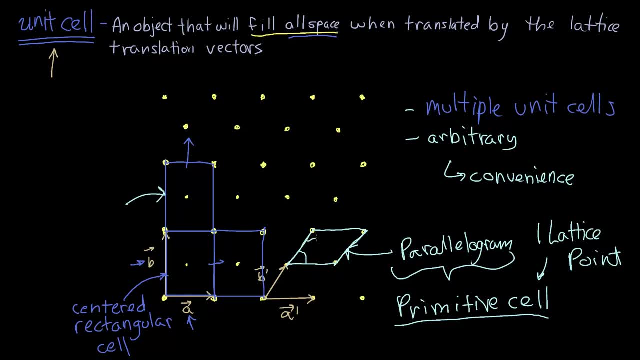 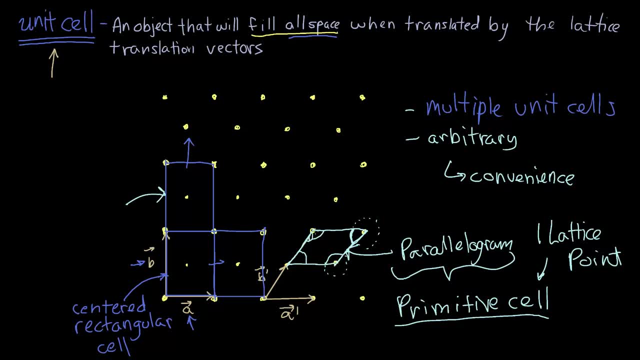 here And you were to add up this contribution from each point, that would give you one lattice point. We could do the same kind of logic on our centered rectangular cell And these guys would add up to two, So we'd have a one quarter here, here, here and here. 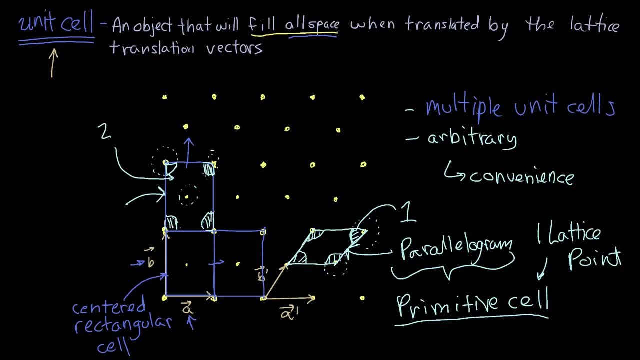 One quarter at each of the The corners of the cell, and then one whole point is contained in the center. This point would not be shared with anyone else. So we have four times one. fourth plus one equals two. The primitive cell is not special really, other than the fact that it has one lattice. 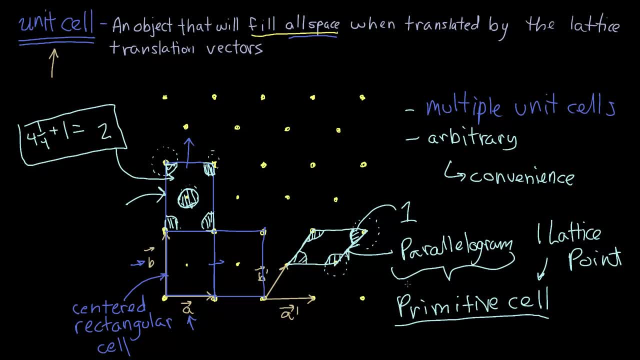 point. In many cases when we go and start working in three dimensions, the primitive cell can look very strange and we tend to work more with cells that have two or more points in them- non-primitive unit cells. A unit cell that I couldn't use would be a circle. 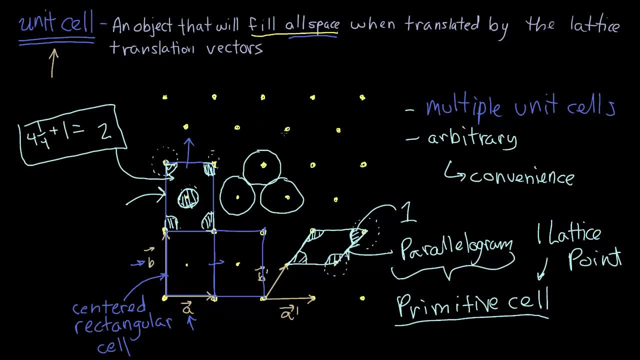 And I'll try and demonstrate that here. So I'll draw some very rough circles around each one of these points And you can see that if I tried to fill space with these points I would be left with some gaps in between. If I tried to fill space with these circles, I should say: 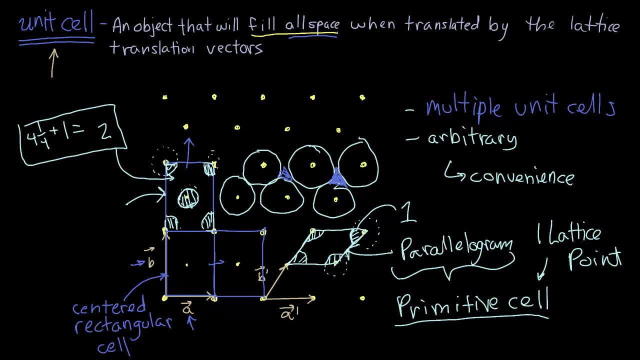 Okay, So. Okay. So these circles would not fill space, Which would break our definition of a unit cell, meaning that circles are not a valid unit cell in 2D space. Analogously, spheres are not unit cells in 2D. 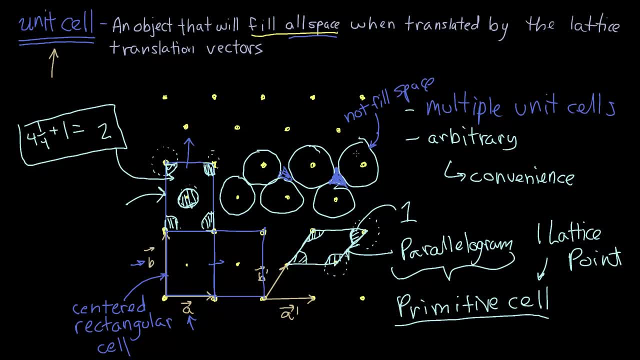 Okay, In 3D space In the next video we are going to work through some examples in. We're going to stick in 2D and we're going to combine our knowledge of the unit cell and the basis and lattice. 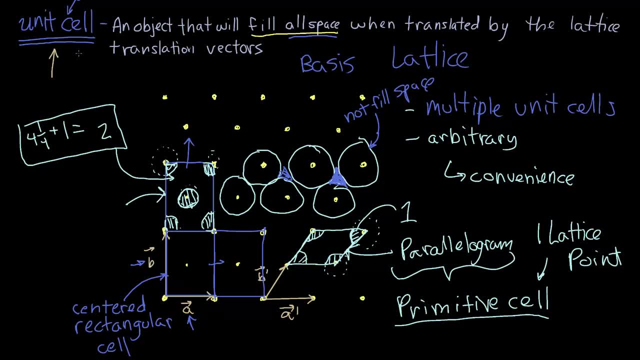 Okay, Okay, Okay, Okay, And we're going to kind of play around a little bit, We're going to get comfortable with these definitions And I hope to see you there.